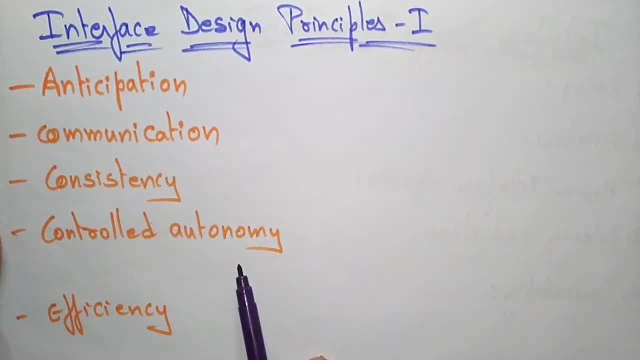 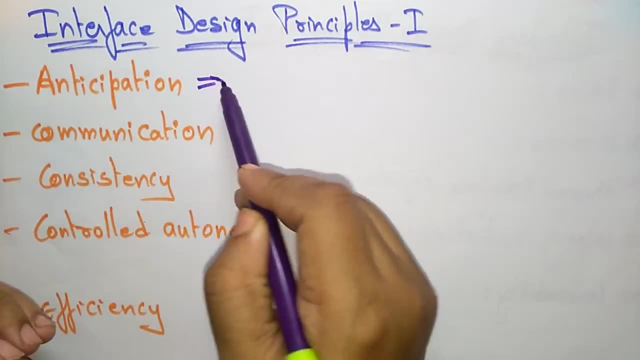 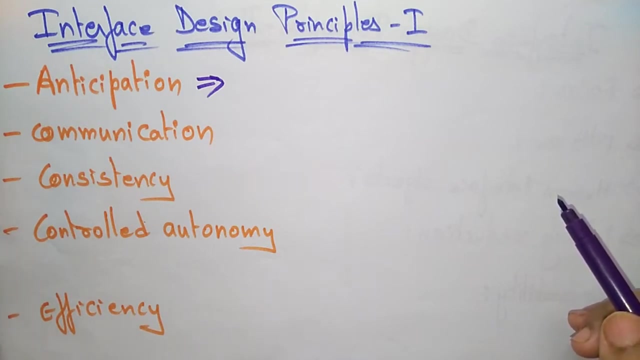 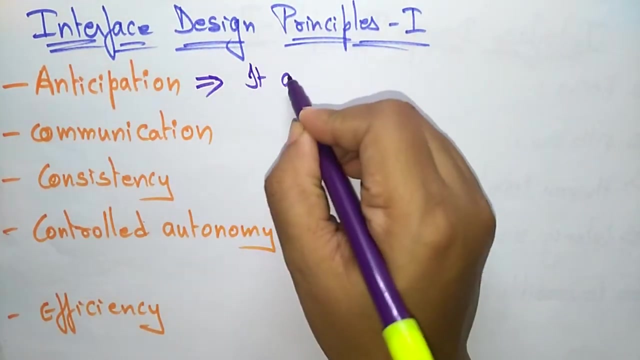 anticipation, communication, consistency, control, auto autonomy and efficiency of that uh interface design. so here the anticipation: a web app. whatever you're going to be created, a web app should be designed so that it anticipates the user's next move. it has to be designed in a way that it has it anticipates, anticipates the user's next move. 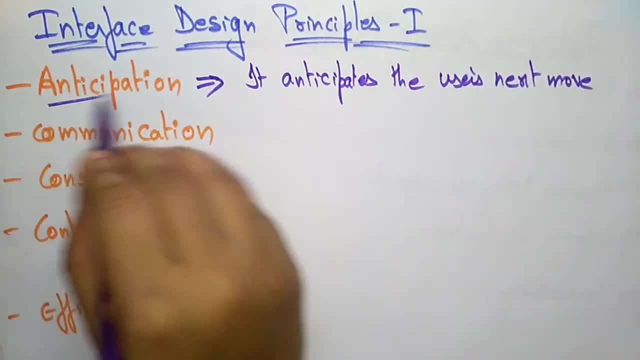 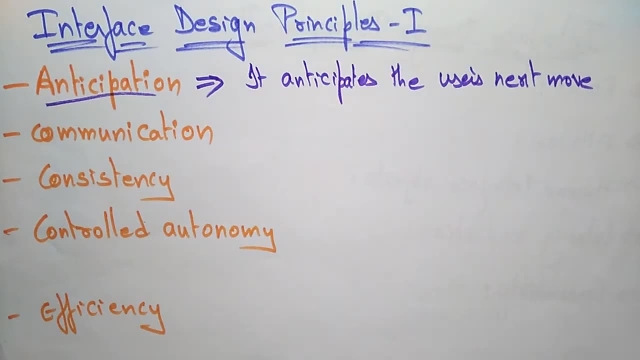 users next move, so that should be identified in your design. okay, so a web app should be designed in a way such that it anticipates the user's next move. then what about the communication here? the interface- whatever the design interface we are using- the interface should communicate the status of any activity initiated. 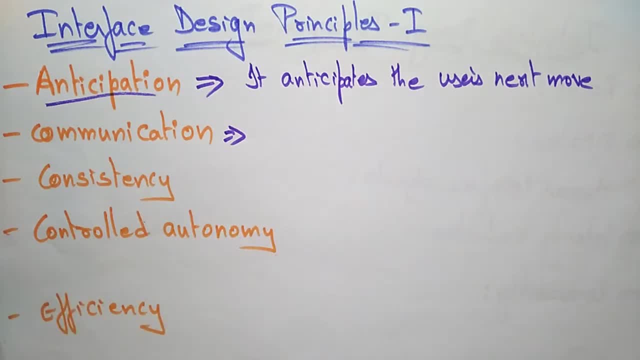 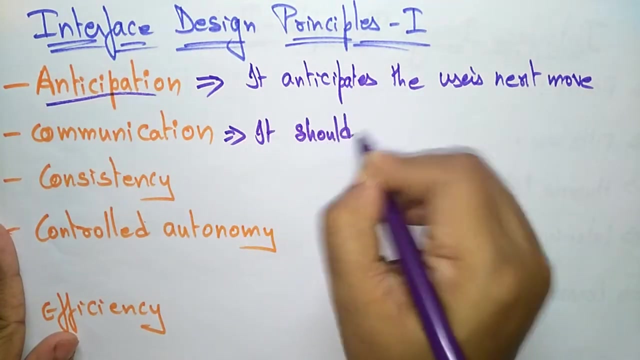 by the user. so the communication is nothing. but we are interacting. to whom? to the users, and the developers and the users are going to communicate with each other. so here, this interface design has to be designed in a way that it should communicate. it should communicate the status of, the status of 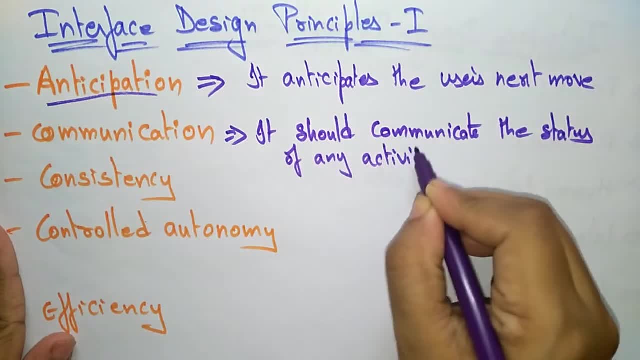 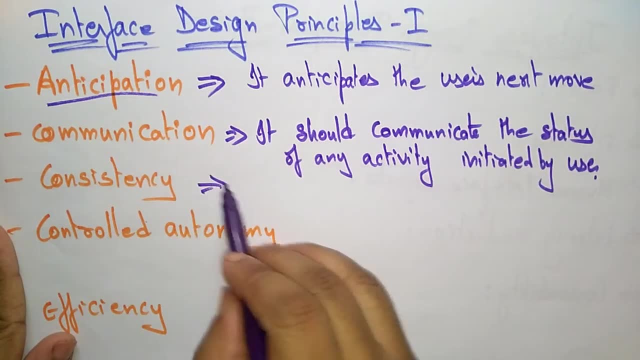 any activity, any activity initiated by user. so, and the next step is the consistency. so, whatever the design you are uh going to develop means, whatever the principal techniques you are following, the main thing is you have to achieve the consistency. so the use of navigations like, let me write that, 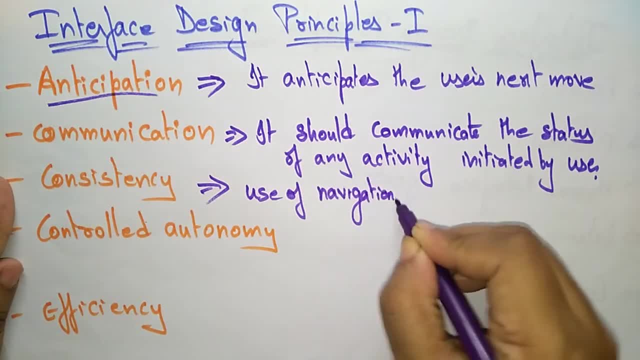 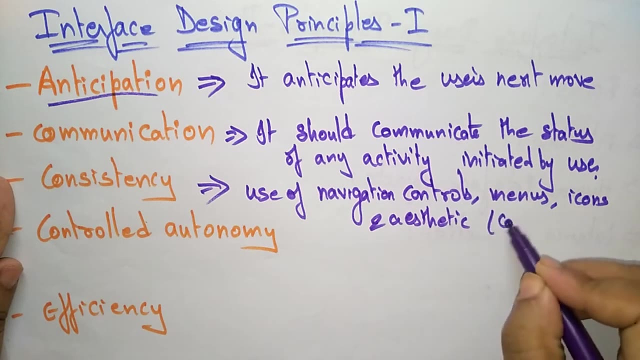 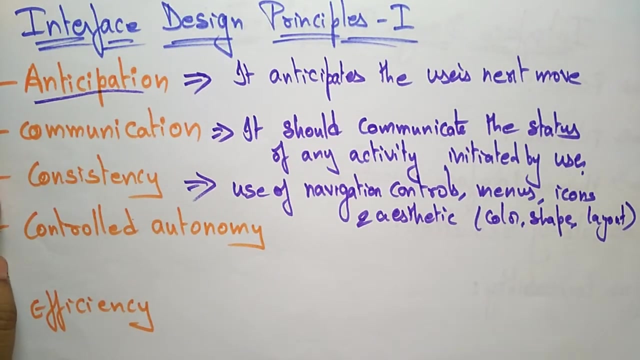 use of navigations. so use of navigation controls, menus, icons and some acetic, uh acetic designs like color, shape, layout. it's just showing the style. the aesthetic design is nothing, but it is just a style representation. so with the help of all these controls you can achieve the consistency. 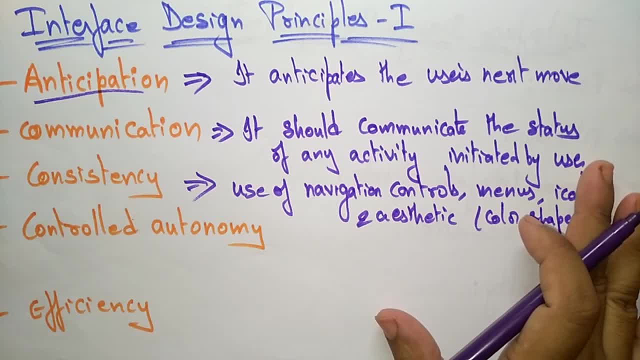 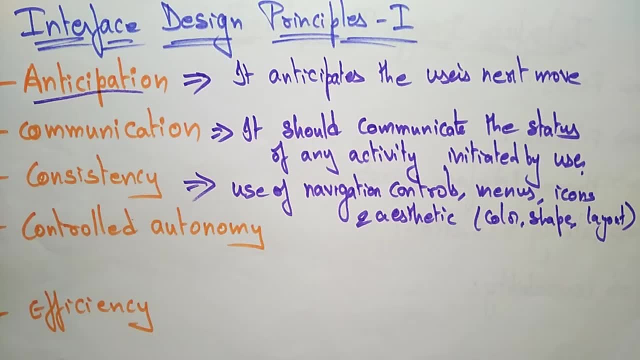 with the help consciously enameth asin design, design, uh, consistency. so how can you say your interface design is consistency? if you use the uh, use the concepts like navigation, controls, menus, icons and color shapes and layout, and if you make it as a understandably, then your interface 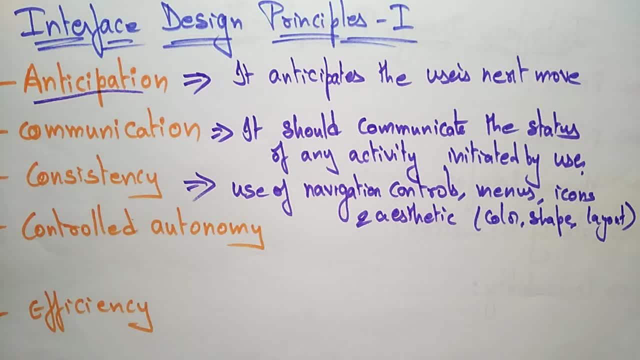 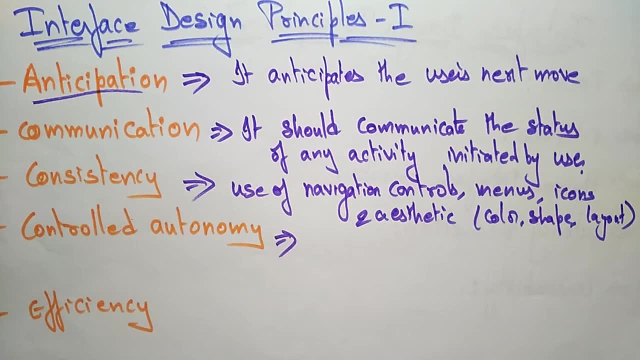 design. it should be consistency. so next one is the control autonomy. so what is this control autonomy? the interface should facilitate user movement throughout, whether isn't it? so the interface should facilitate user movement throughout the web app, so that affects the user. like this is Zum tsch. 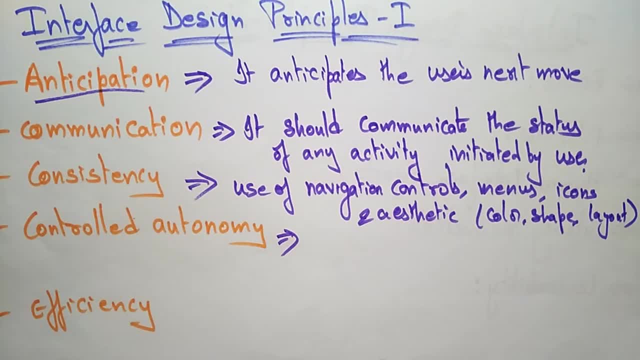 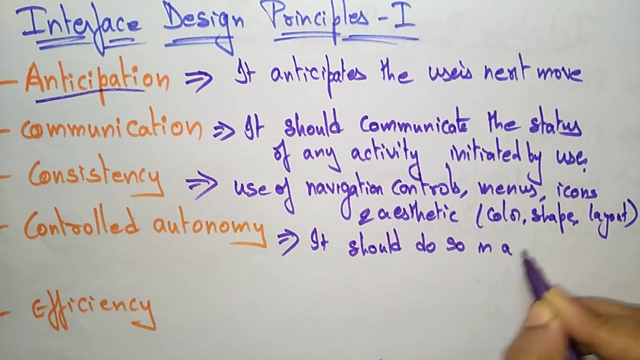 we already know. whatever the interface should facilitate user moment throughout. the web app should be there, but it should do so in a manner that enforces navigation convention that have been established for the app. okay, it should do. it should do so in a manner in which manner it has to be, in a manner that 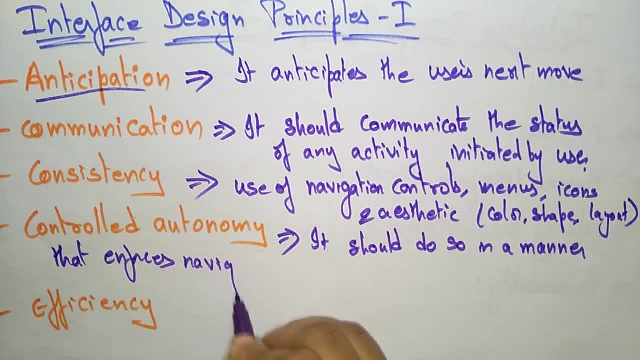 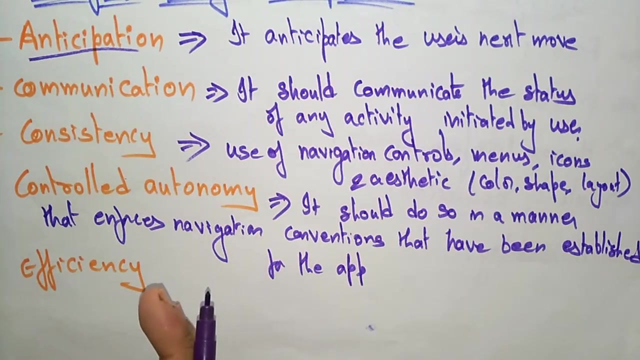 enforces navigation conventions that have been established for the app, and the last one is efficiency. so the design of a bab and its interface, so whatever the interface design you are using, that should be. optimize the user's work environment. so, whatever the interface design you are using, that should be. 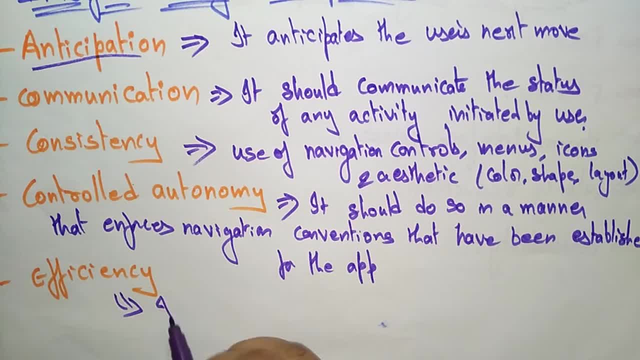 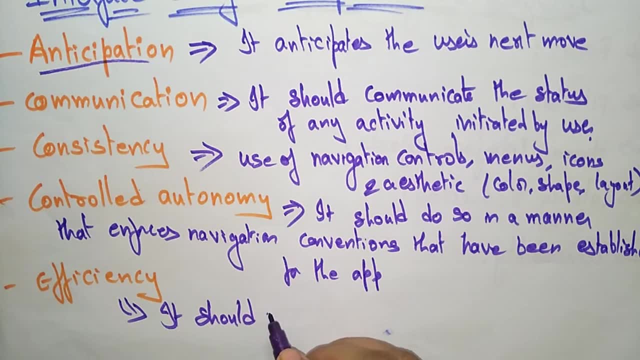 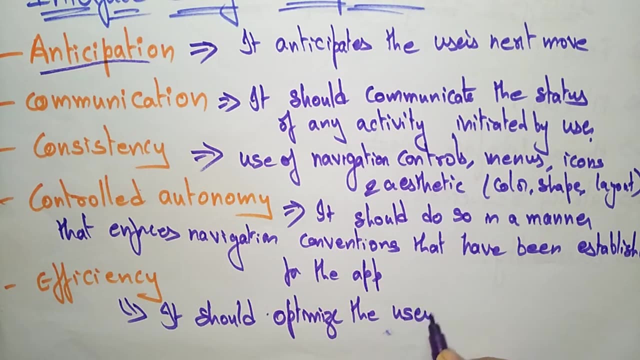 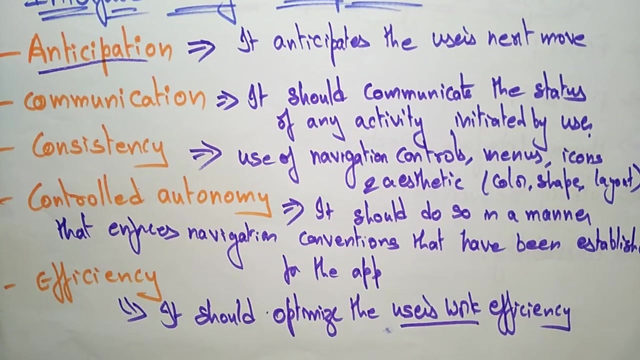 efficiency. okay, the efficiency it should. it means the interface design. whatever you are creating in the web app, it should optimize the user's work efficiency, user's work efficiency. so here we are talking about the efficiency of the user means users are the main persons who are going to use. 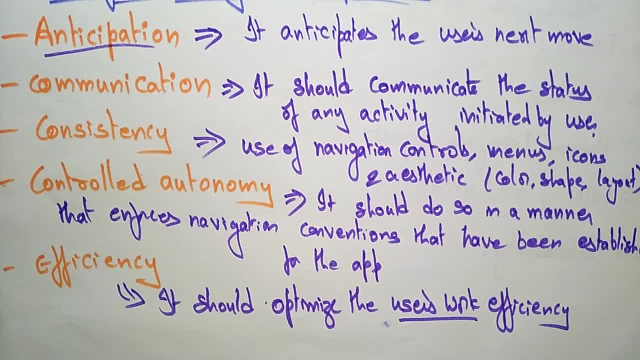 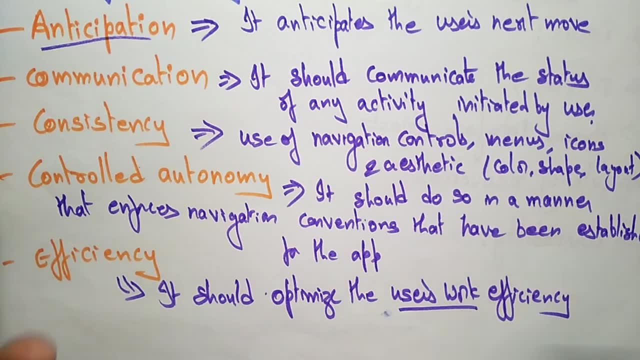 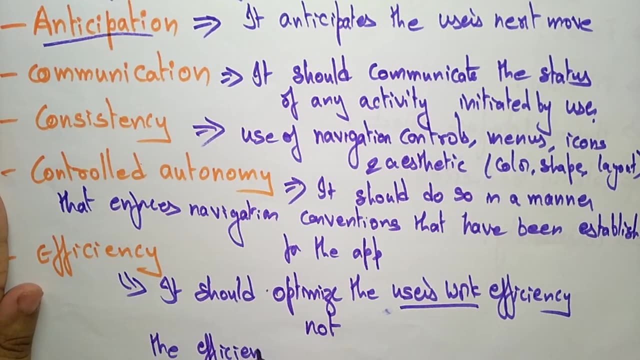 our apps, so they are the customers, means with the uh, with the help of them only we are developing everything. okay. so it should optimize the user's work efficiency, not the efficiency of web engineers, not the efficiency of web engineers or client server environment: client server environment. so if you are going to design, 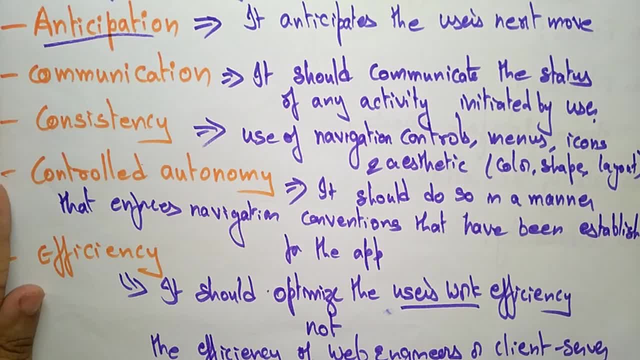 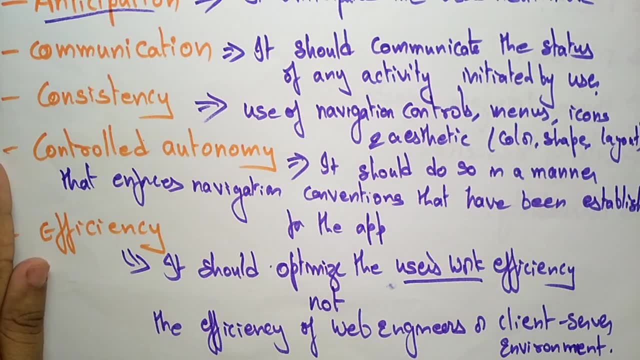 anything. interface, uh, interface design. you have to think about the efficiency, so the efficiency. you have to think in the way of users work efficiency only, but it's not in the way of uh the. you are not supposed to think about the efficiency of web engines or client server environment. so this: